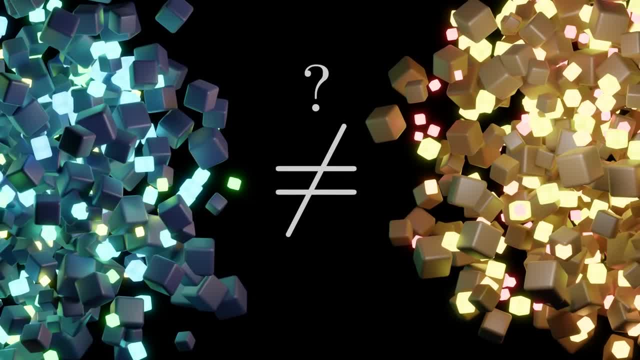 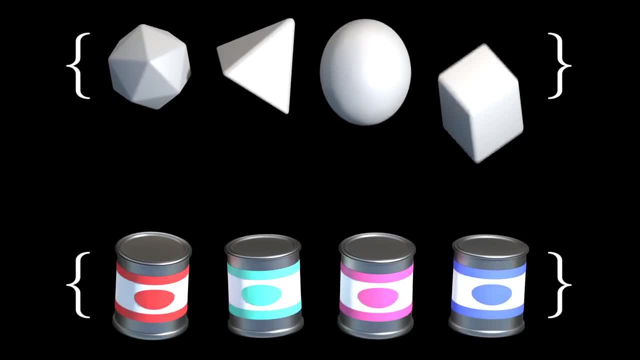 then figure out if it's possible to have two infinite sets with different cardinalities. Notice that if two sets have the same finite cardinality, it's possible to pair each element in the first set with its own personal and unique element in the second set. It's also possible to 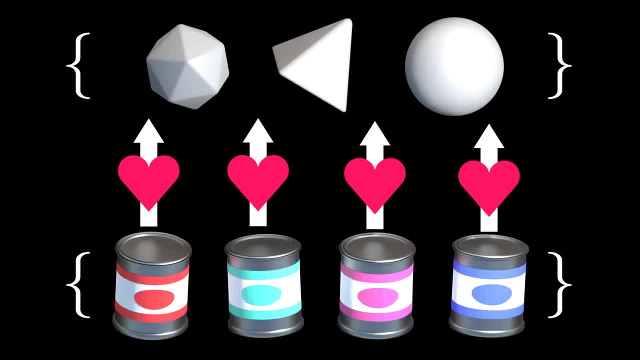 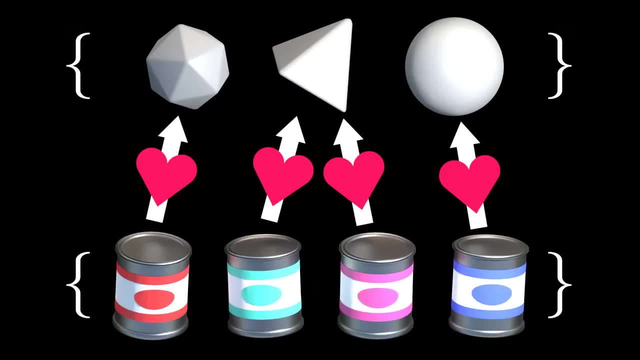 do this the other way around. If the sets have different cardinalities, you can't pair things up uniquely, resulting in complicated love triangles. This is antithetical to many mathematicians' desires to avoid convoluted social situations and is thus contrary to the definition. 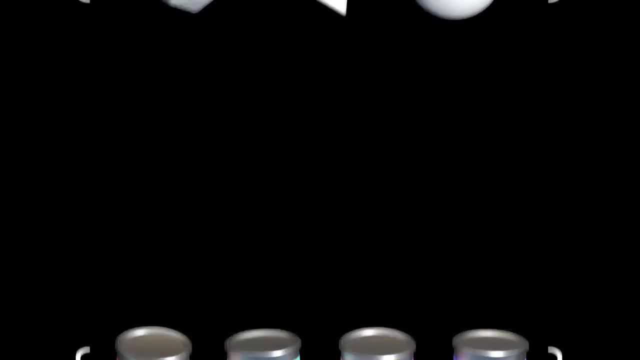 of sets with equal cardinalities. Notice that there's nothing stopping us from trying this property out on our own. Notice that there's nothing stopping us from trying this property out on our own. Notice that there's nothing stopping us from trying this property out on. 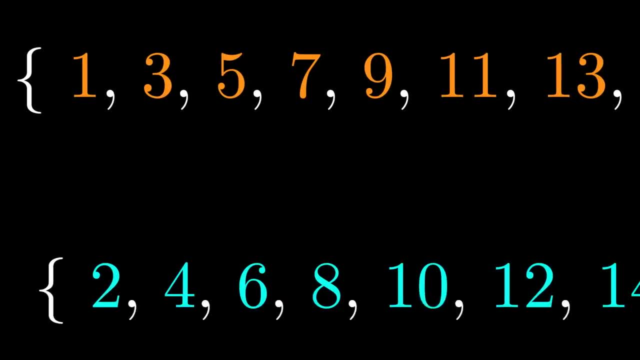 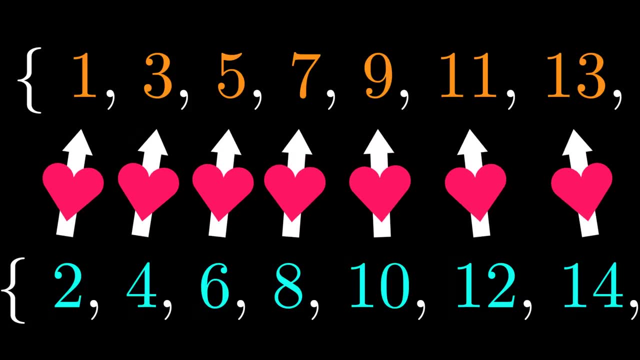 infinite sets. Even though there are infinite odd and infinite even numbers, we can define a pairing between them. It's pretty straightforward to prove that everyone here is uniquely paired up, so they must have equal cardinality, meaning there's just as many even numbers as odd numbers. 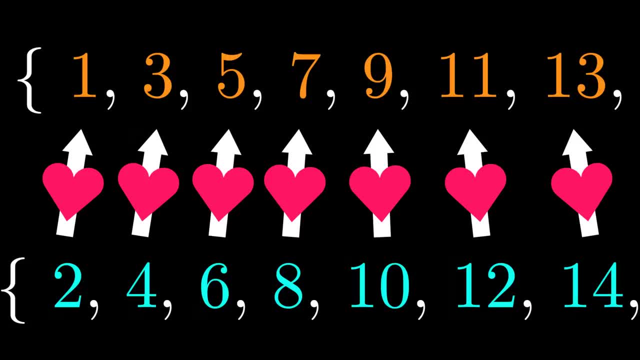 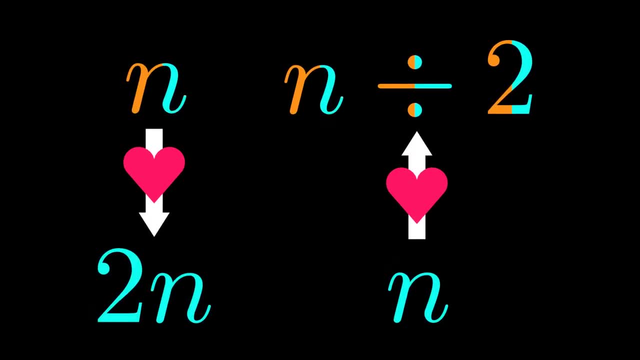 Makes sense. But here's where it gets weird. You can do the same thing between the even numbers and all of the integers. The conversion process is simply to multiply or divide the original number by two. Every even number is paired up with a unique integer. 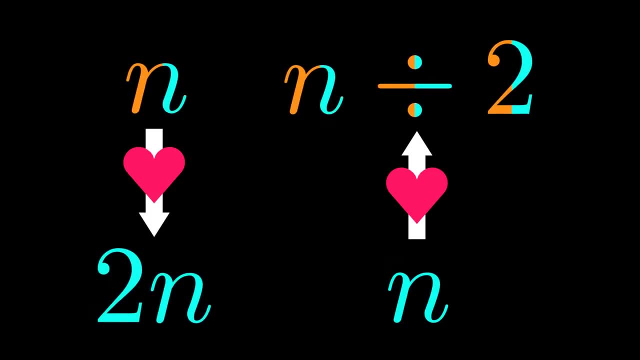 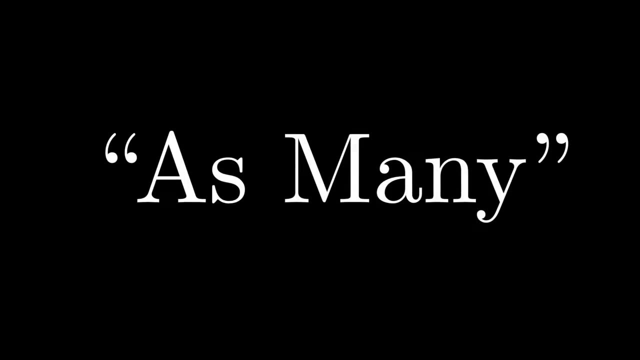 and every integer is paired up with a unique even number, And this is why infinity is so confusing. People will often tell you that there are as many even numbers as there are integers. We use this language because it was the clear language to use when we were talking about finite sets, even though it doesn't necessarily make 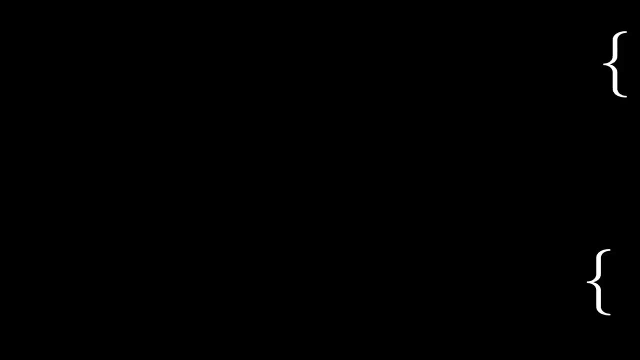 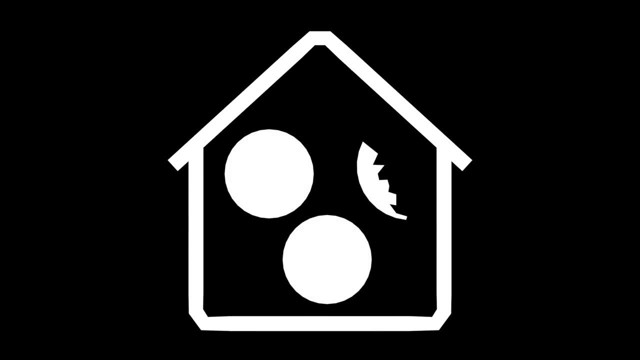 intuitive sense in the infinite case. Using language like this is like saying we're illuminating a surface with a negative light source. It's like saying the average family has 2.19 children. None of these terms make consistent sense and they're not supposed to. 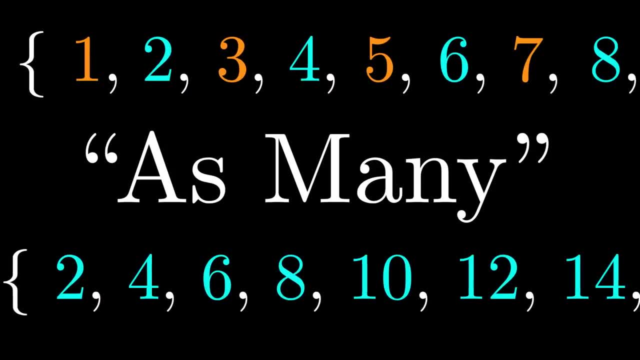 We continue to use the language of the simpler definition when applying it to new cases. But when we teach people about infinity and use these phrases without noting this, we create the false impression that there's supposed to be some kind of intuitive notion of size that works on infinities. The size of an infinite set is an abstract concept. 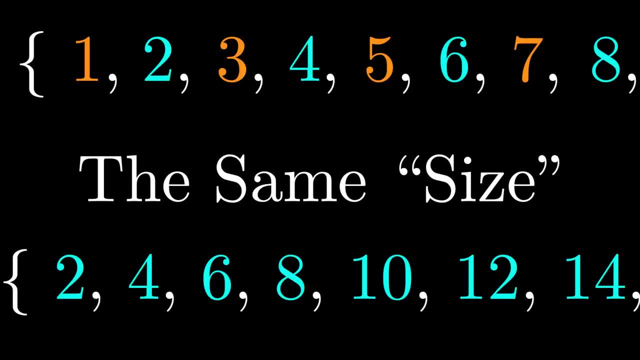 completely divorced from its usage as a term in English. That's why I'm going to continue to refer to this property we're talking about as cardinality instead of size, in the hopes that it helps emphasize that this concept doesn't really work the way the nomenclature of infinity works. So let's get started. 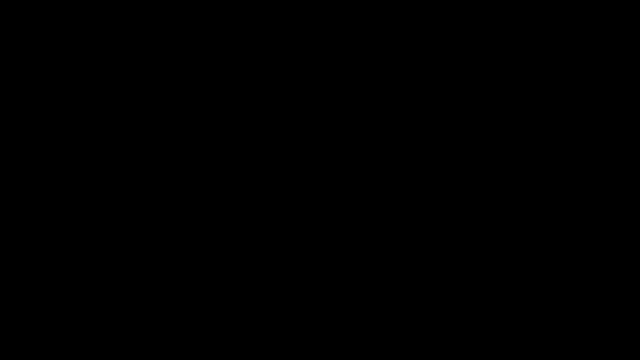 So far it's looking like it might be the case that there's only one infinite cardinality. It kind of makes sense too. If infinity is already bigger than all the other numbers, how can there be something even bigger To confirm this? let's keep trying to make. 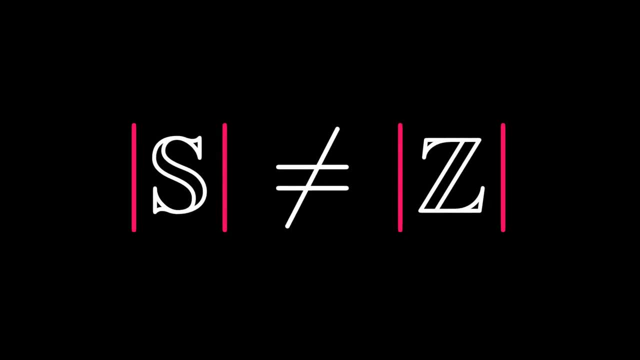 an infinite set that has a different cardinality than the set of all numbers. To start, it turns out that the rational numbers have the same cardinality as the integers. First consider only positive rational numbers. We can order them by starting at 1 over 1, then going. 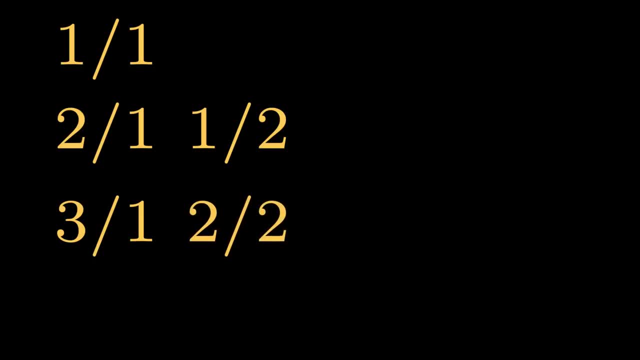 to 3 over 1,, 2 over 2, and 1 over 3, followed by 4 over 1,, 3 over 2,, 2 over 3, and 1 over 4.. Of course, we're going to end up with some duplicate numbers this way. 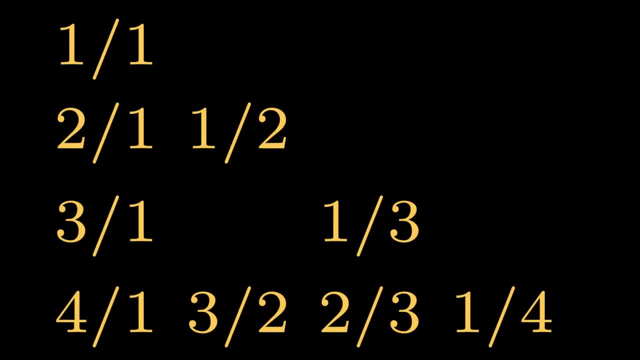 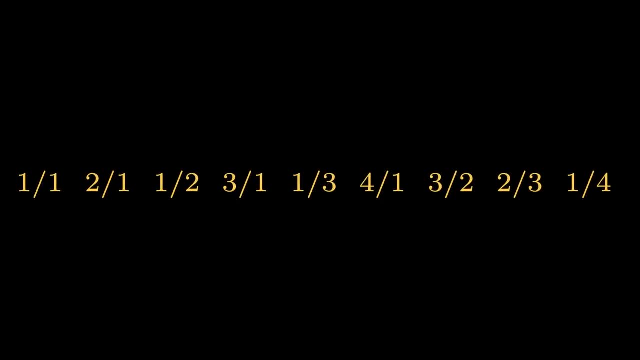 but we can simply skip over those. This process is a way of matching up any positive rational number to a natural number By giving a way to put every rational number in a single file order. we give each rational a corresponding natural and vice versa. We can extend this procedure. 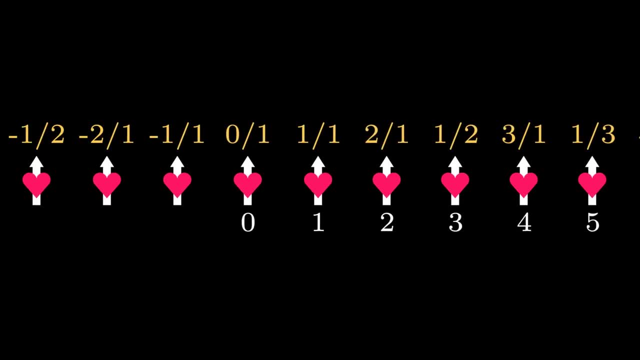 to match up 0 and the negative rationals by simply mapping 0 to 0 and the negative integer to their corresponding negative rationals, Because we can convert between rationals and integers. there are as many rationals as there are integers. If you haven't heard this before. 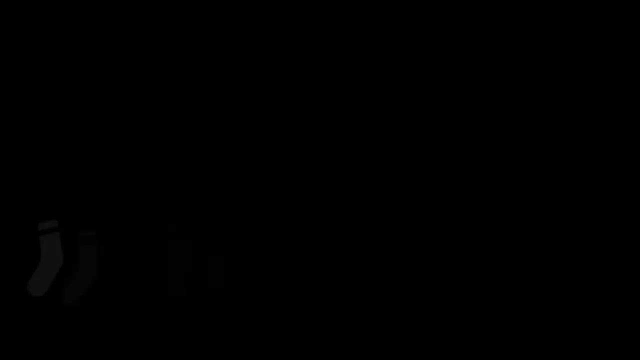 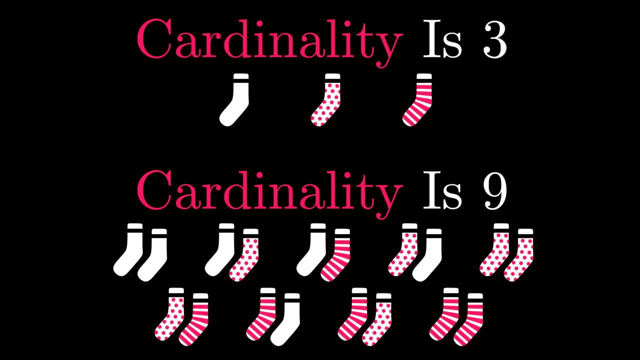 you may find it surprising. Our intuition of size tells us that making all the combinations of elements in a particular set should result in a much bigger set. But since we're unconstrained by intuitive notions of size, we find that it's actually possible to pair up an infinite set of 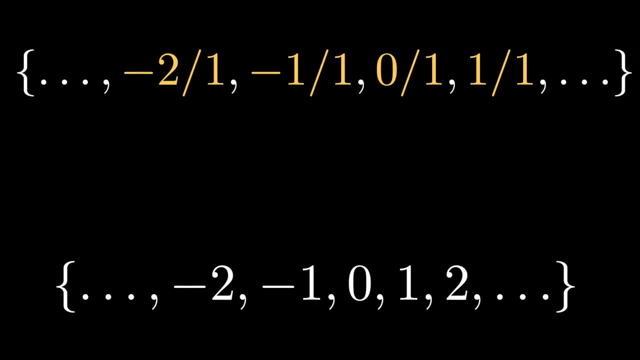 items with an infinite set of pairs of those items. If making this bigger set resulted in the same infinite cardinality, maybe. no matter what we try, we'll always end up with the same infinite cardinality. So let's try one more thing. Let's try making a single file sequence. 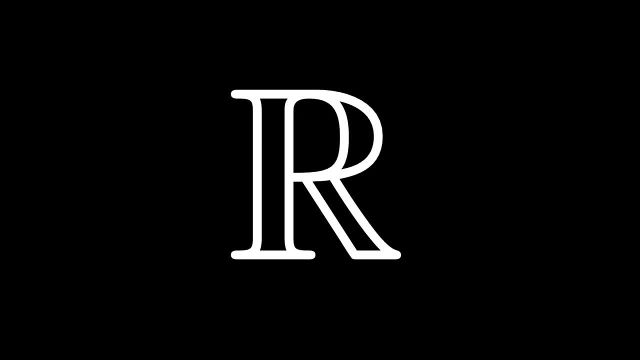 of all the real numbers. Our first idea might just be to try writing out all the real numbers in order. But then which number comes after 0?? Is it maybe 0.1?? But then we've already skipped over a bunch of other numbers. No matter how small we pick the second real to be, there's always. 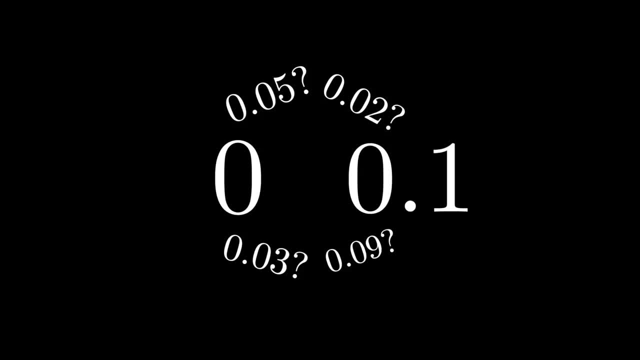 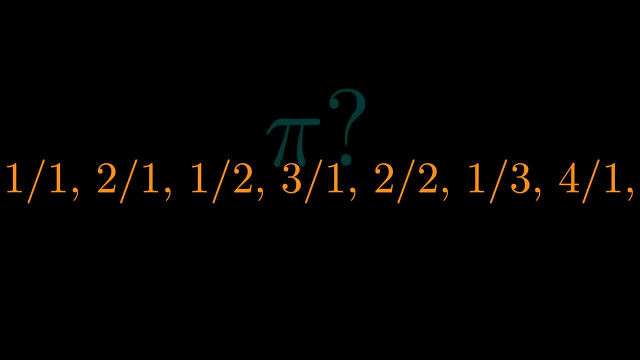 something in between, so we'll always skip over something. So trying to write everything in order doesn't work. We also can't use the trick we use to sort out all the rational numbers, as that would skip over irrational numbers like pi. There's other things we could try to make a 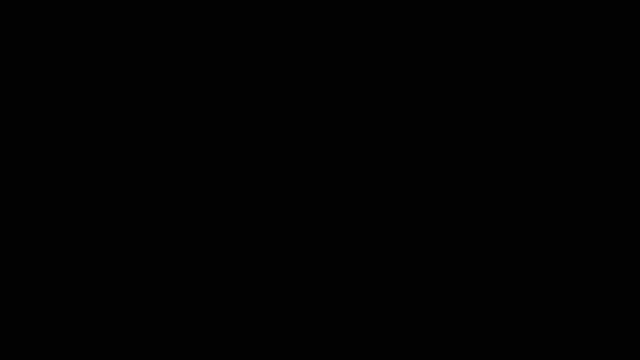 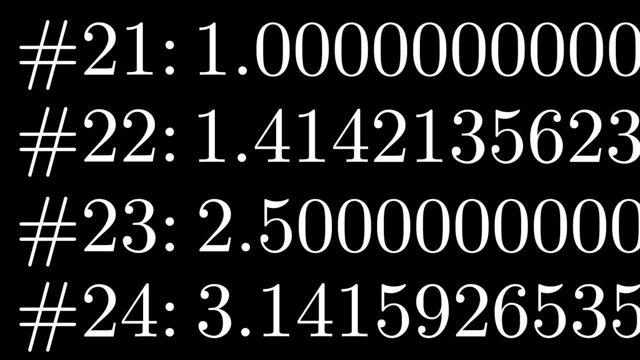 list of all real numbers, but none of them seem to work. It doesn't seem to be possible to make a list of all the real numbers such that every real number gets its own integer number spot on the list. At this point we should stop trying to prove that we can make such a thing and start 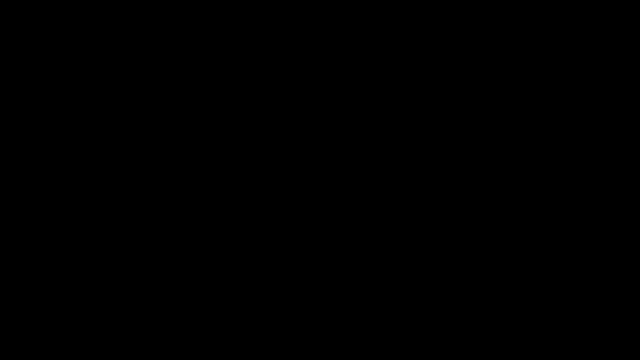 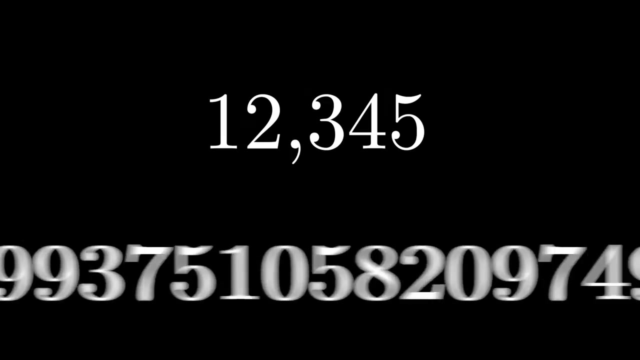 trying to prove that we cannot. An intuitive justification for going down this route is that integers only have a finite number of digits, but all real numbers have a finite number of digits. But all real numbers have infinite numbers of digits. It's impossible to use a finite amount. 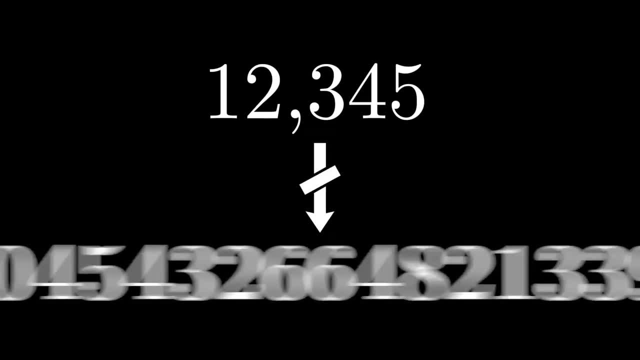 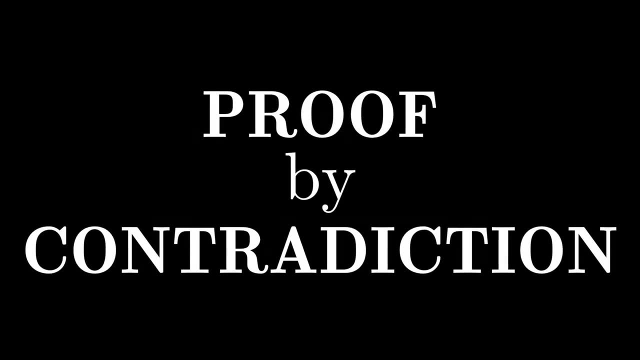 of information to accurately represent an infinite amount of information, so you can't give each real number its own integer. To make a more formal argument, we can construct a proof by contradiction, where we prove that the concept of a complete list of all real numbers contradicts. 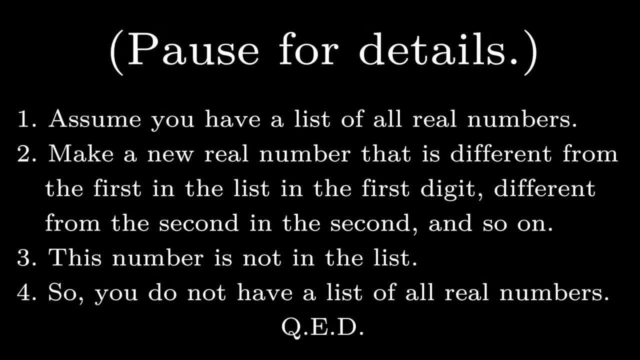 itself. This proof is called Cantor's diagonalization argument, and its generalized version will be helpful to us later. The fact that we can't make a list of all the real numbers finally tells us that there is actually more than one infinite cardinality. So 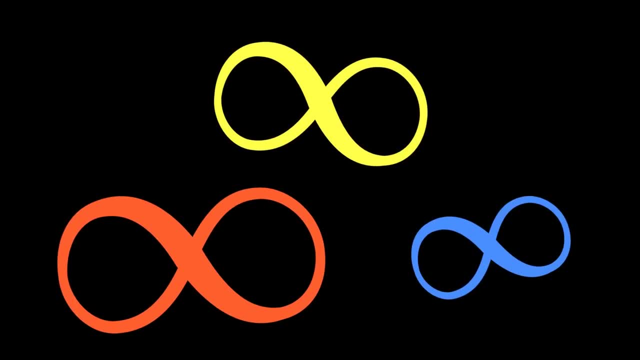 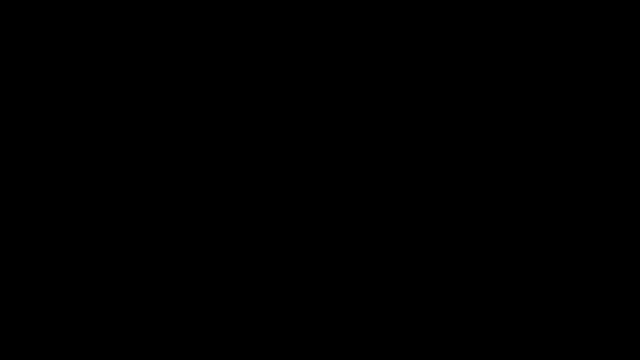 we can't just slap this symbol on these sets and call it a day, Since all the Greek and Roman letters are busy doing physics or whatever. mathematicians invoke the use of Hebrew letters. Specifically, the cardinality of the integers, which is also the cardinality of the naturals and the rationals, is denoted bet0,, while the 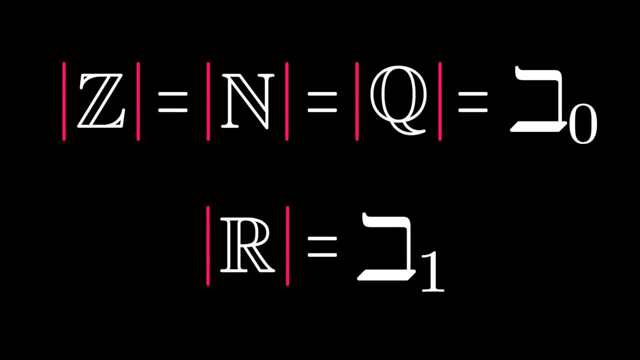 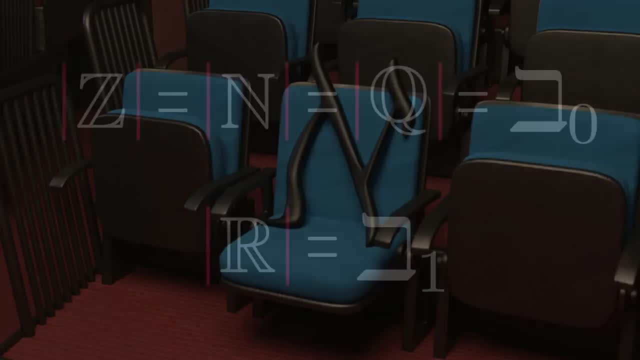 cardinality of the reals is denoted bet1.. If you've heard about this topic before, you might be wondering where Aleph went. They're on break right now, but we'll get into their story once we get to the cardinality of the reals. I'd like to point out that not only are these cardinalities 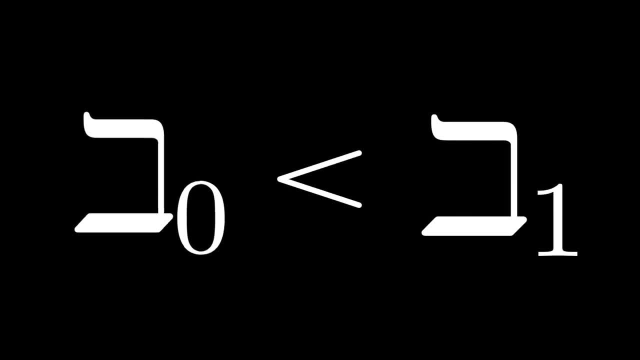 different, but bet1 is in some sense bigger than bet0.. Just like before, we can make a general definition of what this means. that works on both finite and infinite sets. If we have a set with five elements and a set with four, notice how it's impossible to give each of the original elements. 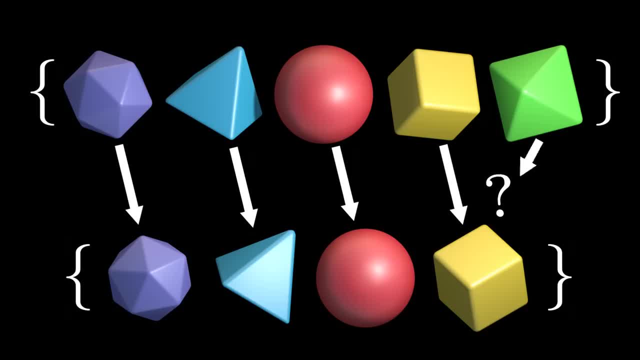 its own unique element in the corresponding set. This means the first set is larger than the second. Notice how this definition is the opposite of sets having equal cardinality. A set has greater cardinality than another one if we cannot make a unique pairing between their. 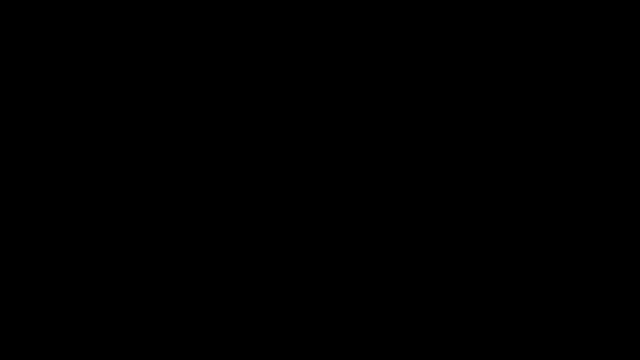 elements. So now we've seen that not only are there many different, infinite cardinalities, but some of them are actually bigger than others. This system of cardinalities is called the cardinal numbers. This name suggests we can do arithmetic to add and multiply cardinal numbers. 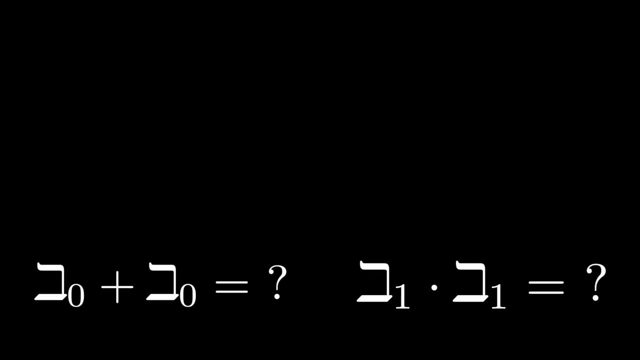 which is exactly what we're about to do. Just like our definition of cardinality, we want our definition of arithmetic to produce the results we expect when we use them on finite numbers, while keeping them general enough to work on infinite numbers as well. 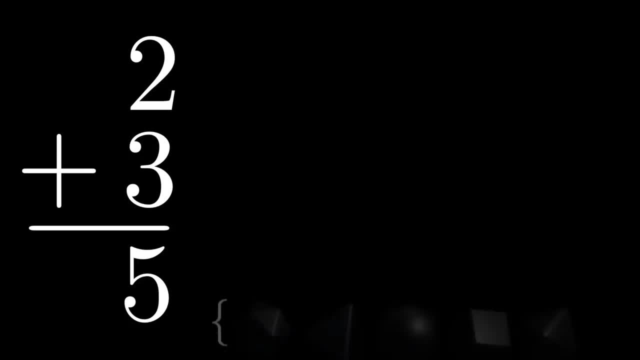 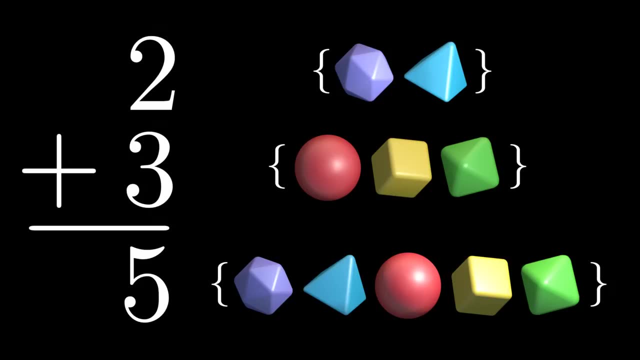 For example, consider this sum. Notice that five is also the number of elements we get if we combine a set with two elements and a set with three elements. In this way we can define what it means to add cardinalities, by defining something to do on the sets, those cardinalities. 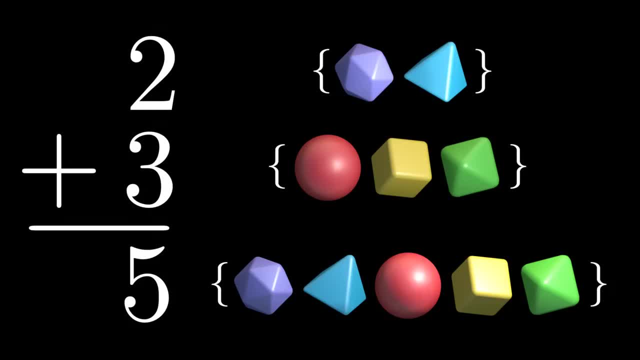 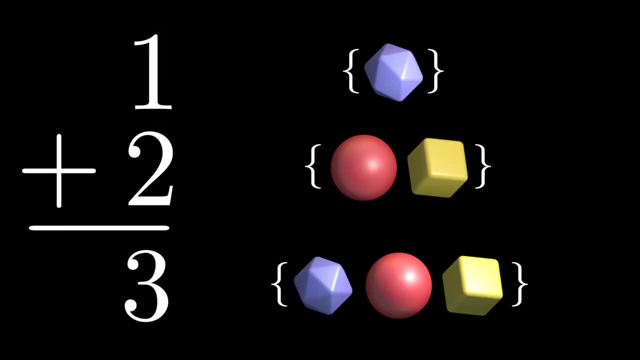 describe. Using this definition, we get an operation that behaves exactly like conventional arithmetic addition for finite numbers, but we can apply it to infinite numbers as well. For example, we can find the value of bet zero plus one by finding the cardinality of. 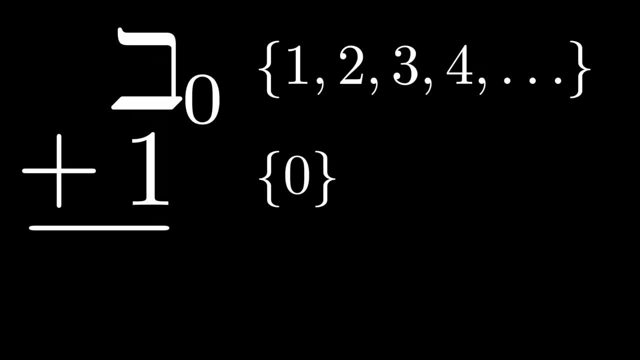 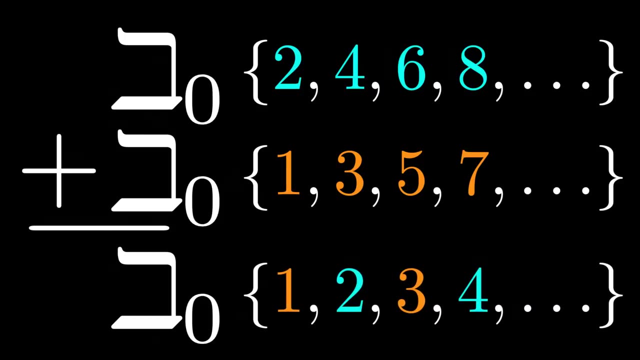 the natural numbers with zero. thrown in The value of bet zero plus one afterwards is just the non-negative integers, which also has cardinality bet zero. So bet zero plus one is bet zero. Similarly, we find that bet zero plus bet zero is still bet zero, because combining the even and odd numbers gives us the natural numbers. 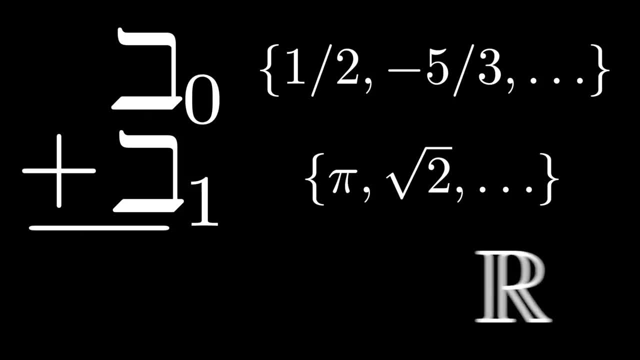 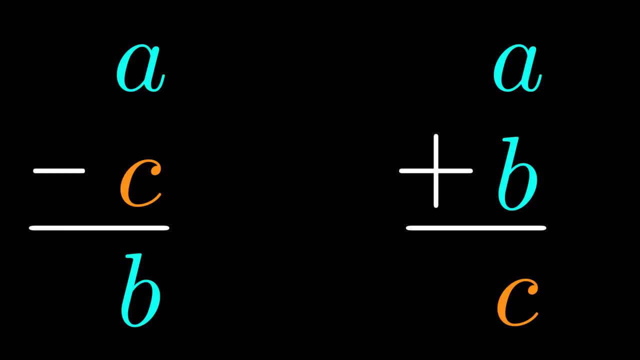 Finally, bet zero plus bet one is like combining the rationals with the irrationals to get the real numbers. so we get bet one. Now we can define subtraction as the operation that undoes addition, But this is a bit tricky, As we've seen. 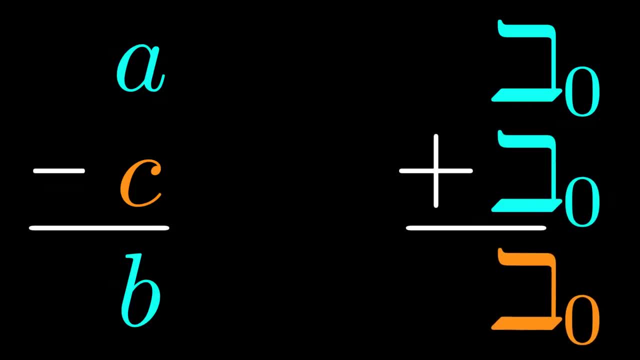 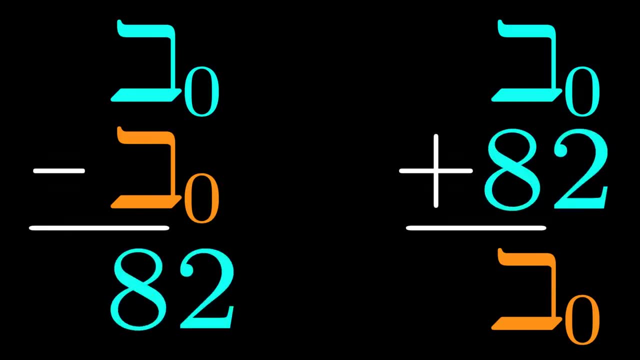 we can't just say that the value of bet zero plus one is bet zero, but bet zero plus itself is also bet zero. That means bet zero minus itself could be one, or it could be bet zero, or it could be any number of things. But you've probably seen something like this before in the 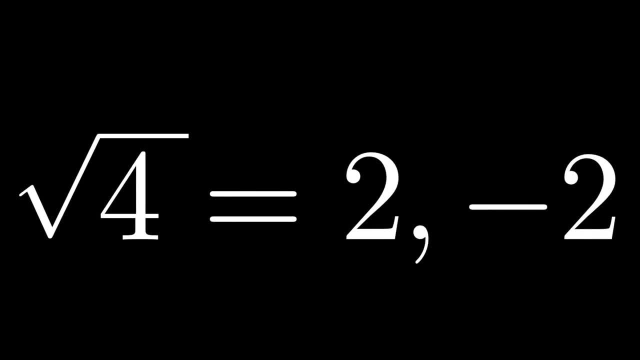 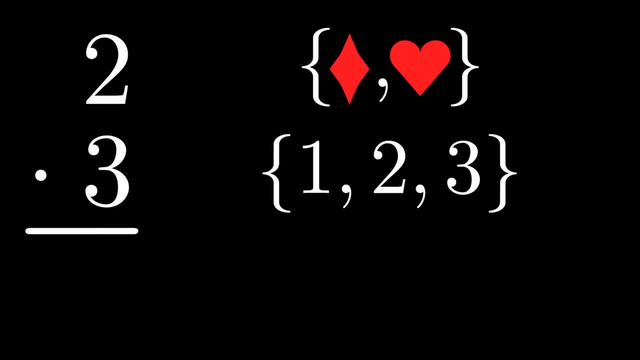 form of square roots. Remember that the square root of four is not just two, but also negative two. We simply acknowledge that the expression in question refers to multiple values and make sure not to treat it as if it is unique. Multiplication is defined as the cardinality of a set containing 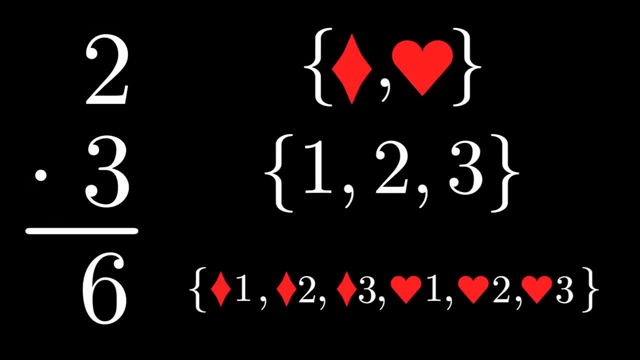 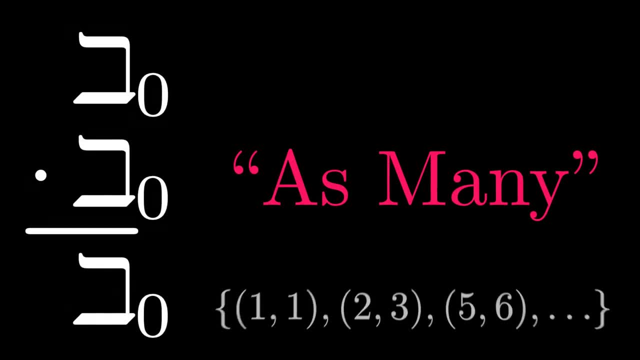 sets. So two times three is six. Interestingly, bet zero times itself is still just bet zero, Similar to what we did with the rational numbers. there are as many pairs of natural numbers as there are natural numbers themselves. Bet one times itself is also bet one. 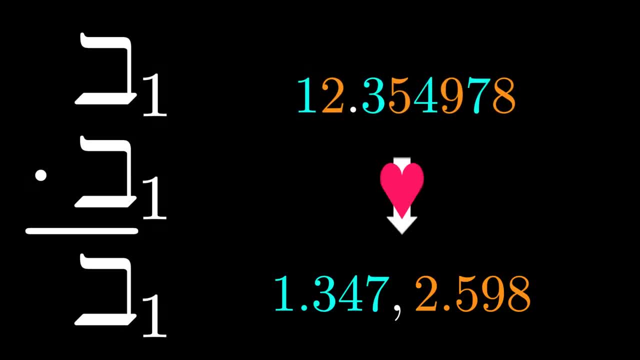 Every pair of real numbers can be assigned its own unique real number and vice versa, so the two sets must have equal cardinalities. You can perform this assignment by taking any pair and interleaving their digits to get a single real number. Deinterleaving lets you go the other. 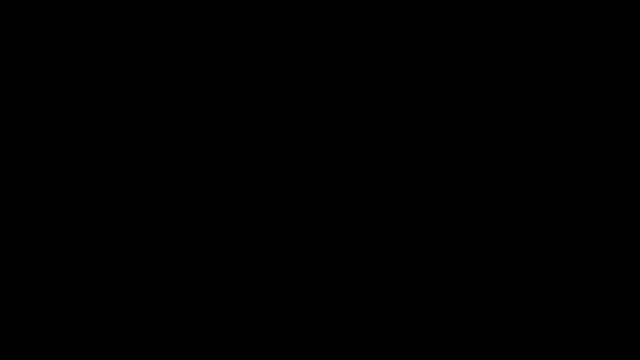 way assigning real numbers to pairs. Finally, raising two to the power of a cardinal number has an interesting interpretation on its corresponding set. If we take a set with two elements, we can recombine those elements into four different sets, while three elements 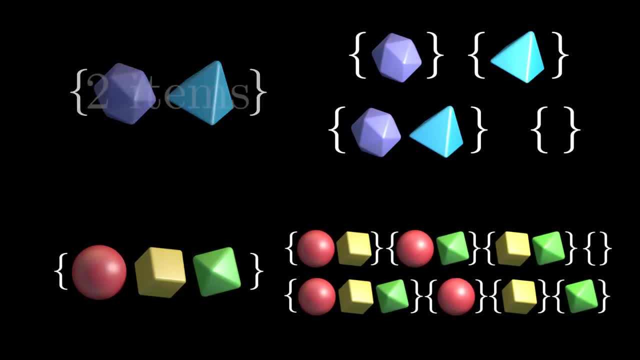 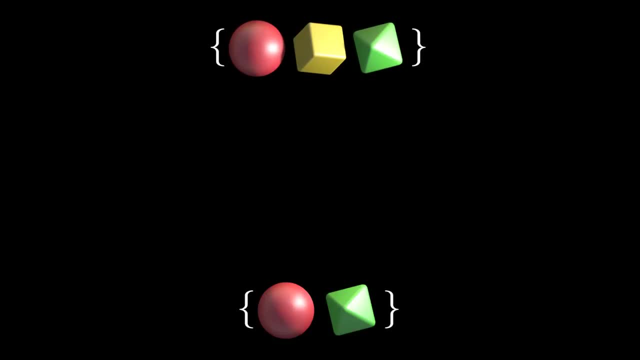 can be recombined into eight different sets. Notice that in both cases we've ended up with a corresponding power of two. This is because, when we have three elements we can choose to put in, every set represents a unique combination of three yes or no decisions. So 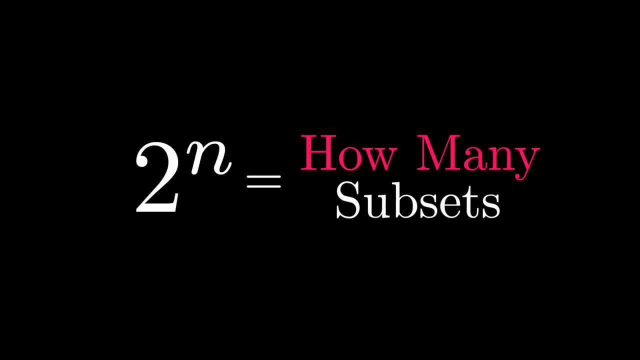 raising two to the power of a cardinal number gives us how many new sets we can make only using elements of the original set. Previous operations seem to leave transfinite numbers intact, resisting any attempt to make bigger ones. This operation fixes that. Two to the power of bet zero is now finally bet one, Actually. 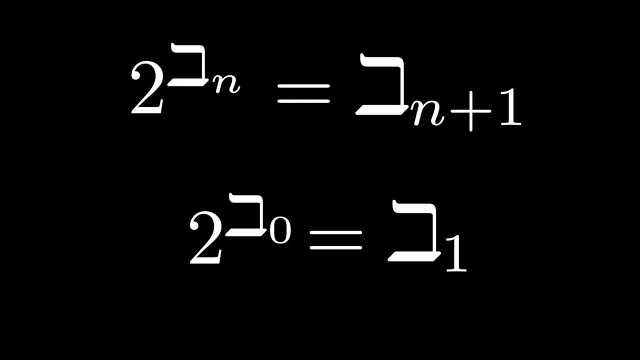 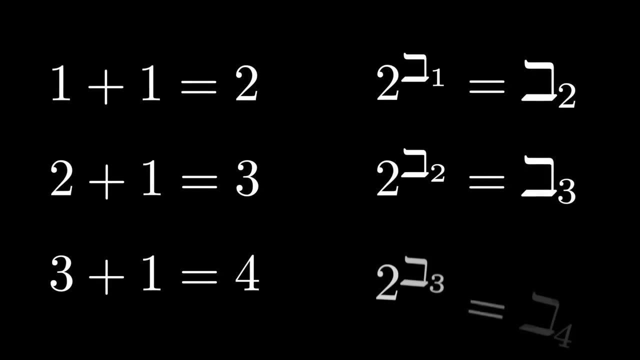 this is the definition of the bet numbers. We can use the diagonalization argument I mentioned earlier to prove that this always results in a distinct and bigger cardinal number. Just like we can repeatedly add one to get bigger and bigger finite numbers, we can repeatedly raise two to a power to get bigger and bigger transfinite numbers. 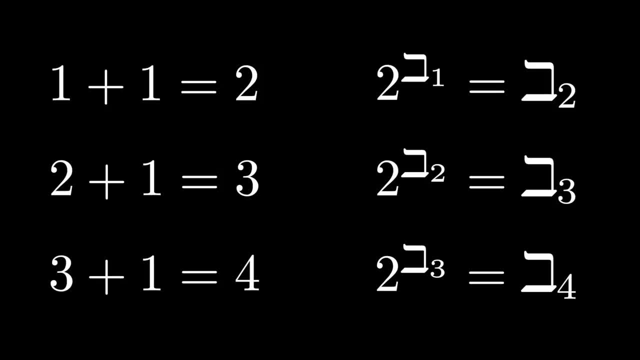 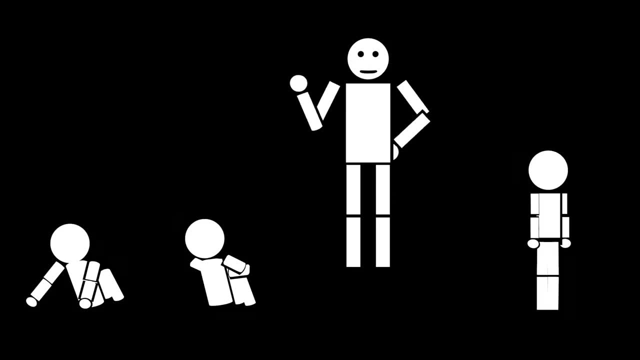 I do find it kind of funny that we need to resort to such a brute force operation to get anything bigger at all. Can you imagine if we did the same thing with natural numbers? Alright class, let's practice our numbers. One, two, four, sixteen, sixty-five thousand five hundred thirty-six. 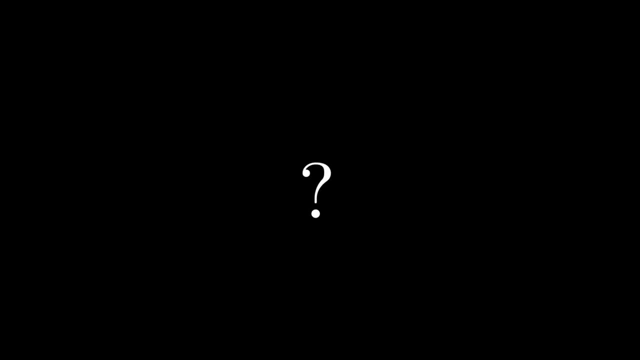 Now a reasonable question to ask is whether or not there's a cardinal number between bet zero and bet one. This is where our friend Aleph comes in. Aleph zero denotes the first cardinal number, which is also bet zero, and Aleph one denotes the next bigger cardinal number after that. 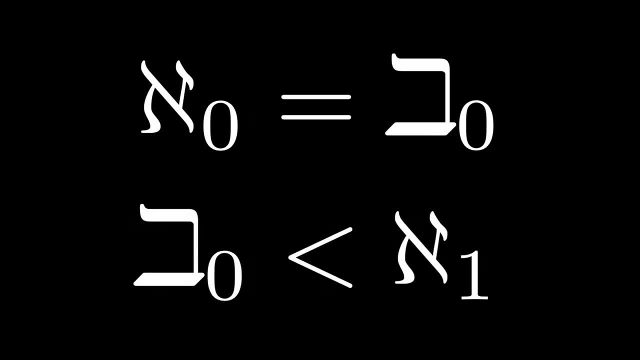 In other words, it's a cardinal number that is greater than bet zero, while leaving no room for another cardinal between them. A reasonable guess is to say that Aleph one is just bet one, that the real numbers come right after the rational numbers. 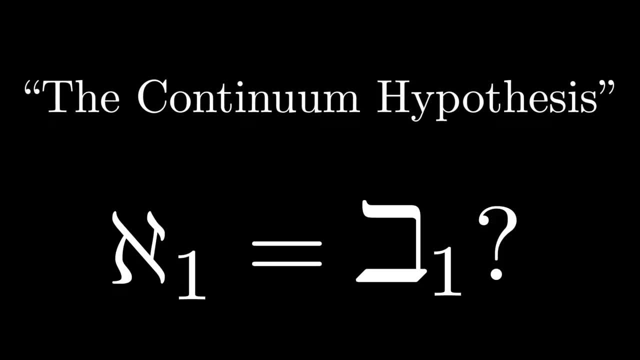 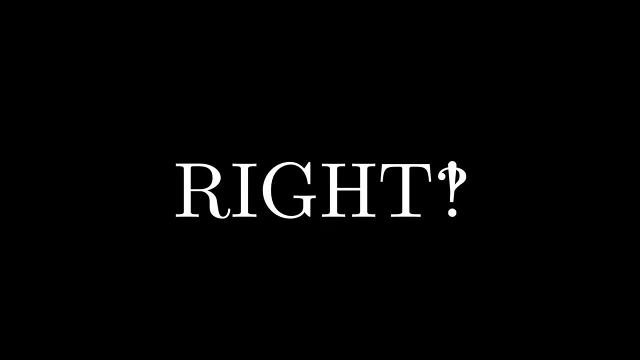 This conclusion is called the continuum hypothesis. While a bit headache-inducing to think about, it sounds like we should be able to prove it true or false with a clever proof. right, Right, But no, This question is not just hard to answer, it's literally impossible. 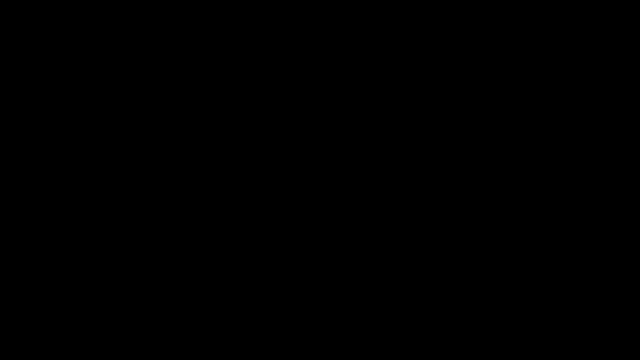 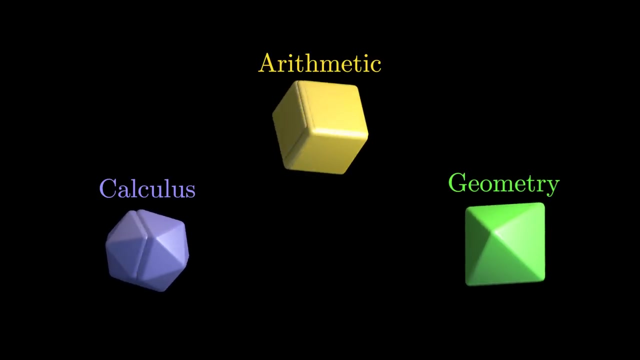 To fully appreciate this, we're going to do a little history lesson. Back in the early 1900s, math was going through a bit of a crisis. At the time, different areas of mathematics were all based on different assumptions because they all talked about different kinds of objects. 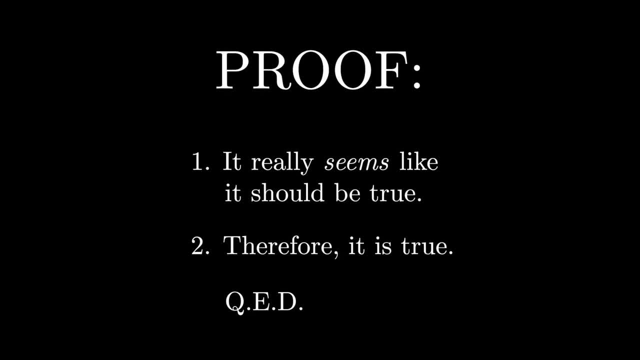 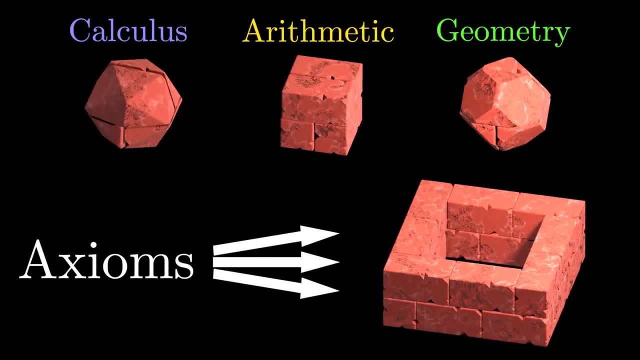 Many proofs relied on intuition for some steps rather than formal arguments. Some mathematicians built a unified system of starting assumptions, called axioms, which could be used to rigorously describe all other fields, but these attempts failed for one reason or another. Usually, 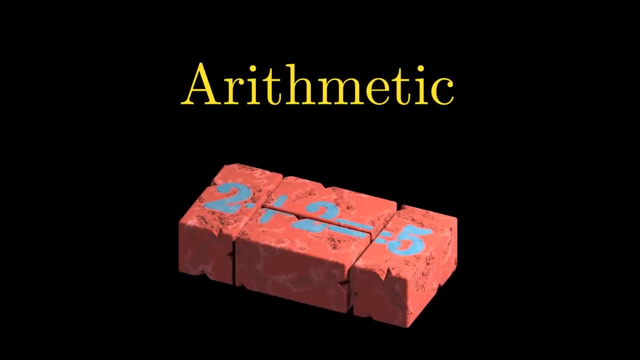 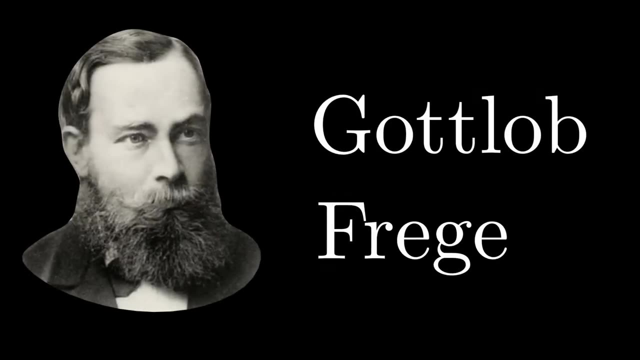 the axioms allowed you to prove a statement that would be considered obviously false, with the existing systems of mathematics rendering the new system useless After ten years. mathematician Gottlob Frege was just wrapping up the second of two volumes on a system of mathematics he defined. 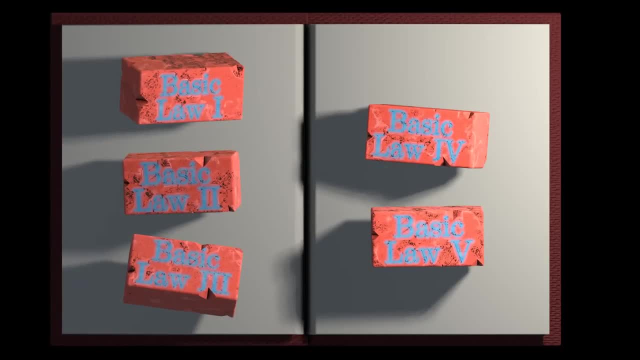 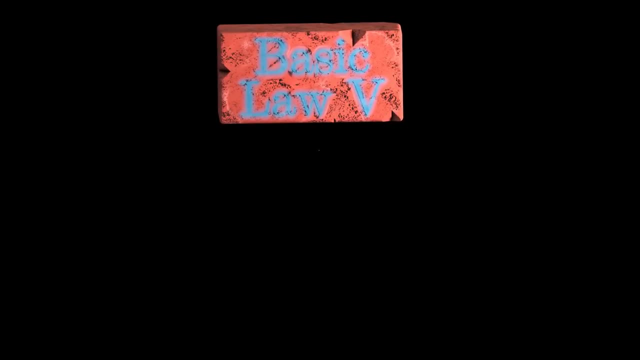 using axioms he felt were intuitive and obvious. As this book was just about to become available to the public, another mathematician informed him that one of his axioms could in fact be used to construct a famous paradox published just two years earlier. This implied that truth. 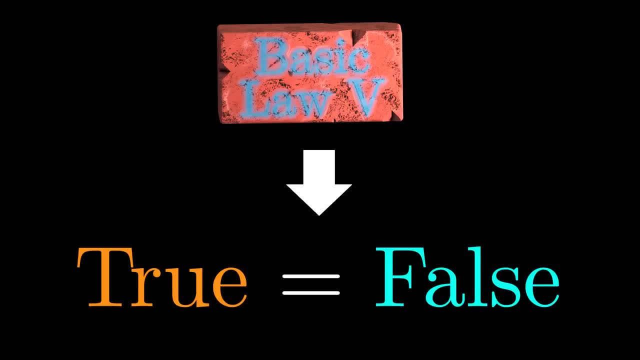 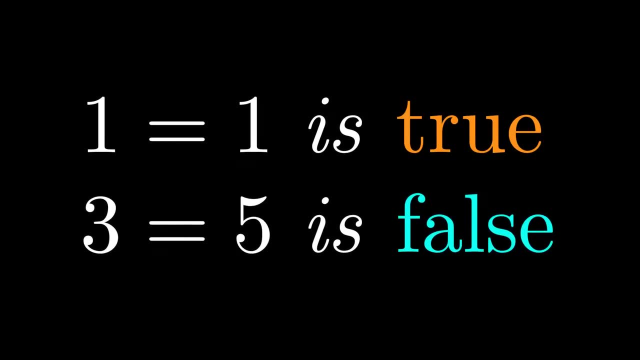 and falsehood, as defined in the system, were actually the same thing. Technically, there were no contradictions in the system, because it's always valid to say that a statement is true or false. It's just that, due to this paradox, everything is true and false at the same time, so 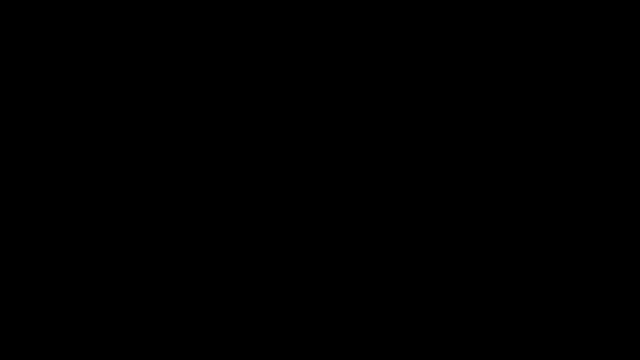 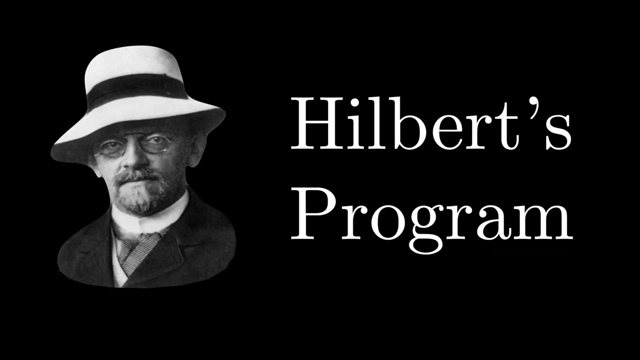 the concepts lose their meaning. Into this unfortunate situation entered mathematician David Hilbert and his program. David Hilbert and his program- Hilbert's program- was his personal vision for what a unified system of mathematics should include. Among others, it included goals such as: we should prove that the system we come up with 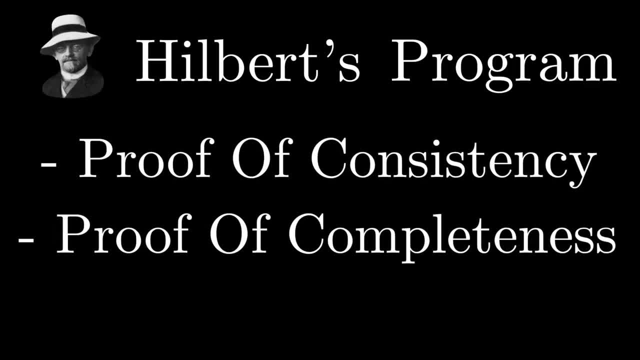 can be trusted because it has no contradictions. We should prove that anything that is true can be proven with the system. It should come with an automated way to check the truth of simple mathematical statements, And these would all be very nice things to have. It would clear up all. 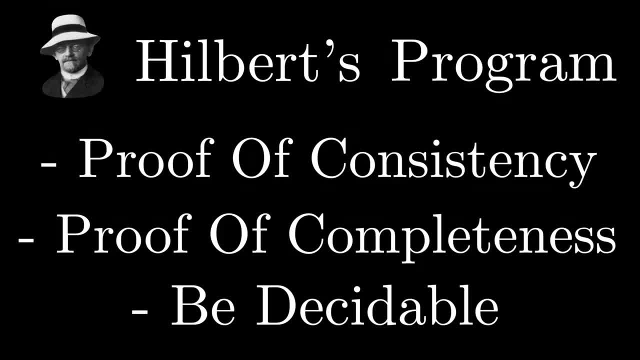 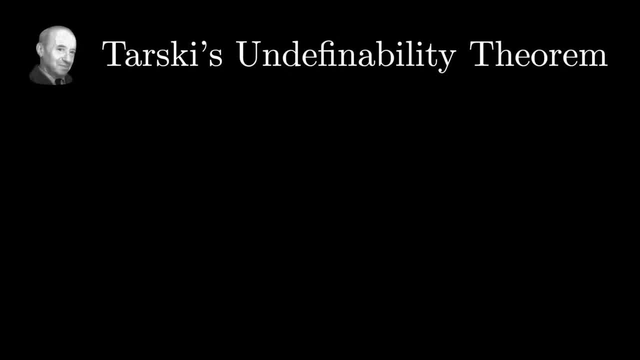 the problems they had at the time, But unfortunately a number of seminal proofs completely obliterated. Hilbert's program Tarski showed that you can't make a formula for telling the truth or falsity of a statement. If you could, there's nothing stopping you from using that formula in a new statement. 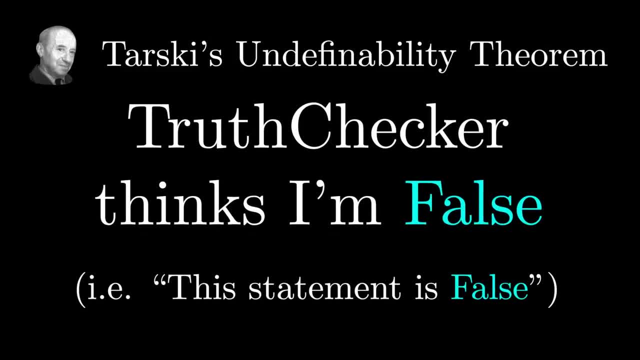 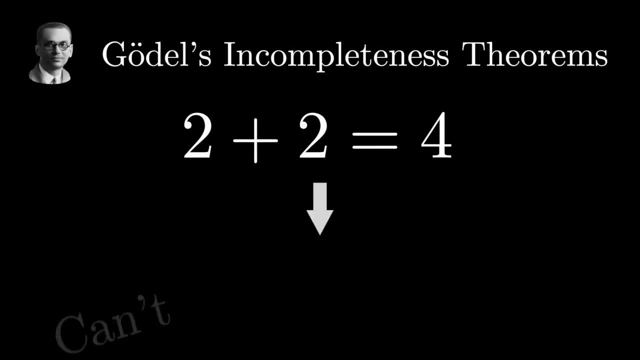 specifically, which the original formula by definition cannot accurately answer. And then this guy named Gödel comes along and says that if your system can do even basic arithmetic, it can't prove everything. And to top that all off, he proved that one of those unprovable statements 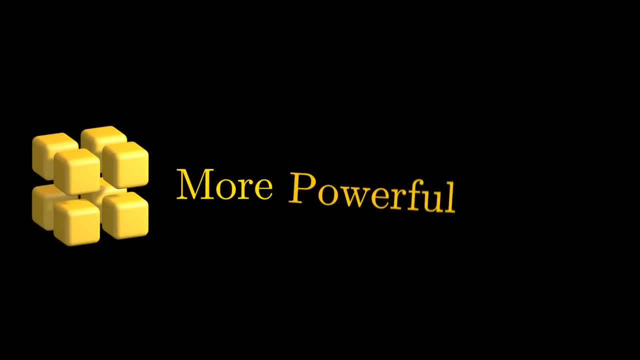 is whether or not the system is trustworthy. You'd have to come up with a more powerful system to answer that question. You'd have to come up with a more powerful system to answer that question, But then you don't know if the more powerful system might have its own contradiction. 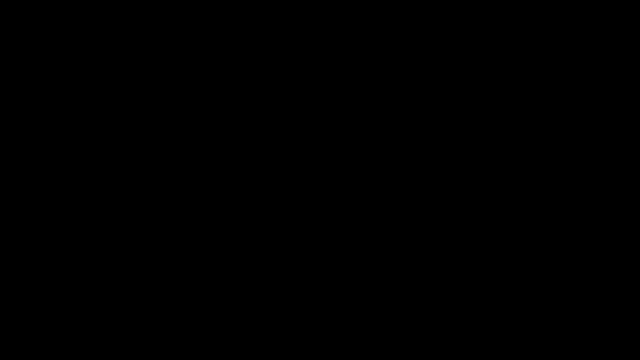 Once everyone got over that load of disappointment, they eventually settled on a good enough system of mathematics called ZFC. It might contain a lurking contradiction, but so far no one's found one, so it's probably fine. Maybe this is okay, Maybe we just accept. 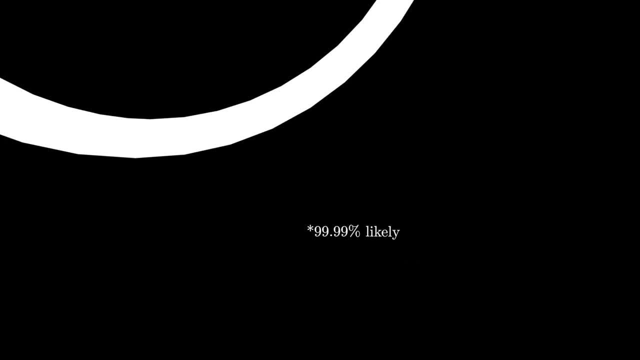 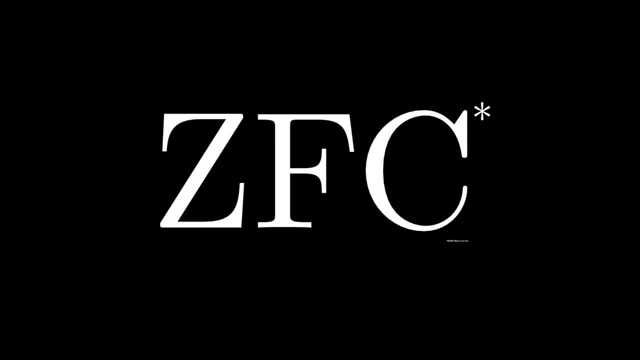 that everything in math comes with a little 99.99% likely to be true. That's better than most everything else. Even though we can't prove there's no contradictions, we can basically prove everything. here's not true if it makes sense. 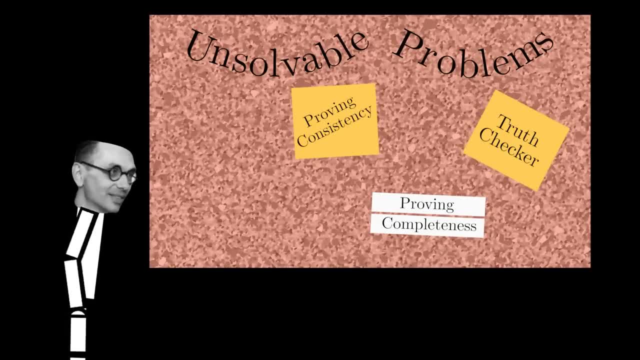 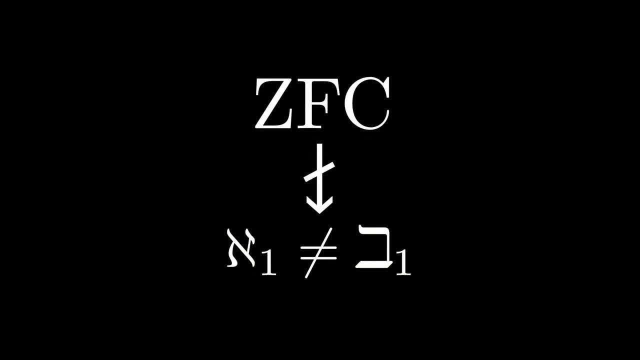 To be specific, the ZFC system isn't strong enough to prove or disprove the continuum hypothesis. if you try to make a stronger system, you could always design it so that the continuum hypothesis is true, or you could design it to make it false. Mathematicians have shown a few statements to be equivalent to the truth or falsity of the continuum hypothesis. So, basically, how true these are depends on how you're feeling, on any gave feeling on any given day. Luckily, though, these results are relatively inconsequential. 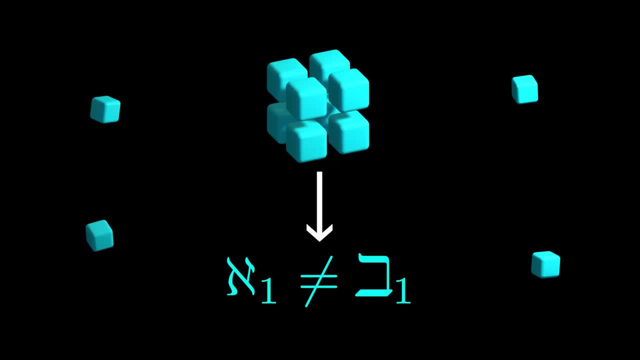 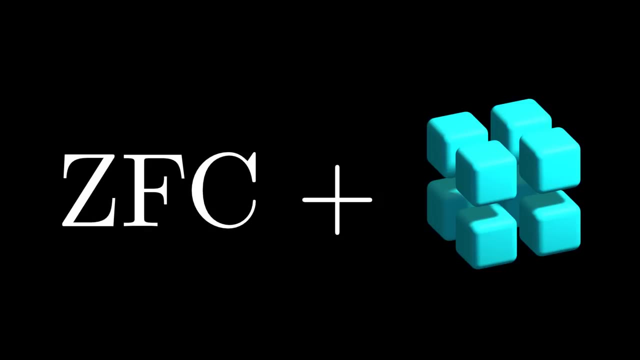 and we haven't found any practical use for them Yet, Which is why no one's bothered to rally an effort to officially extend Z of C, to accept or reject the Continuum Hypothesis. What's much, much worse is this C? See, it used to just be ZF, but then mathematicians 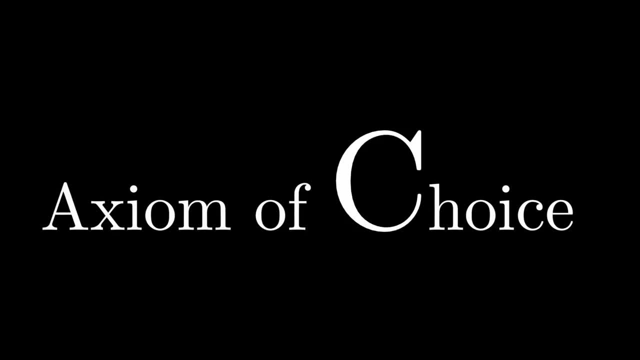 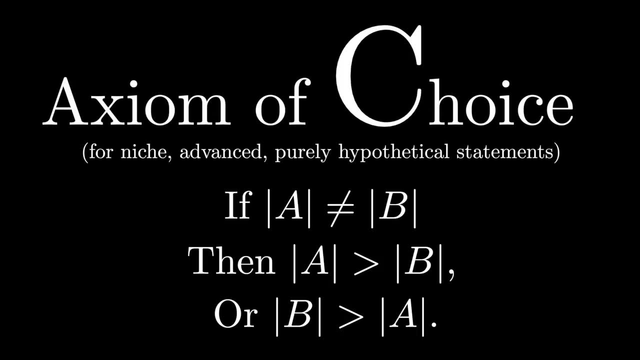 realized it would be really handy to have this thing called the Axiom of Choice, so that they can prove a few niche-advanced, purely hypothetical statements like if two sets aren't the same size, then one of them is bigger. Luckily though, math seems to favor. 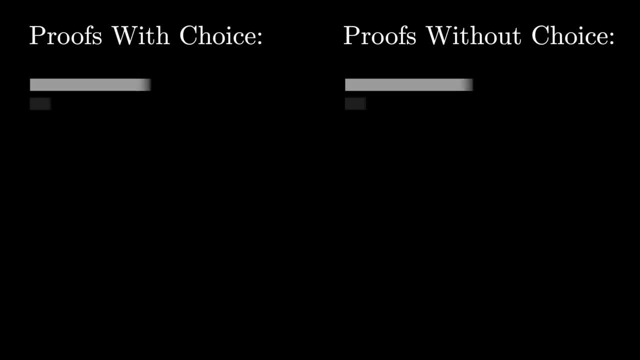 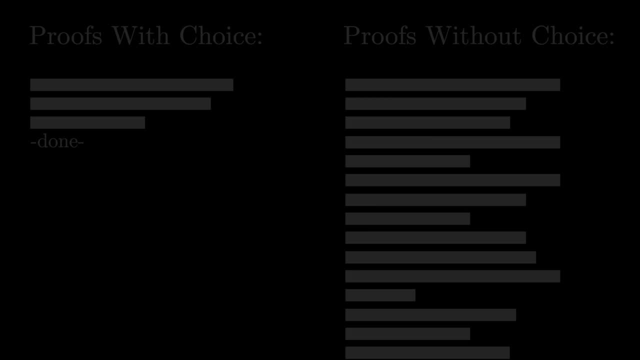 it being true much more than it favors it being false. Math is just more cumbersome to do without it. Well, that's the end of that tangent. Let's get back on track and finish learning about how infinity works. The one thing left to wrap up is what infinity? 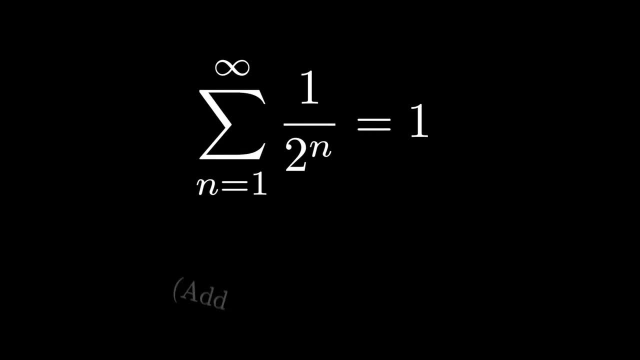 means in these kinds of equations. Informally they mean you should do the operation forever until you get a single answer. But this definition doesn't really work. The definition of the function, for example, requires adding together a bunch of numbers until you get an answer. 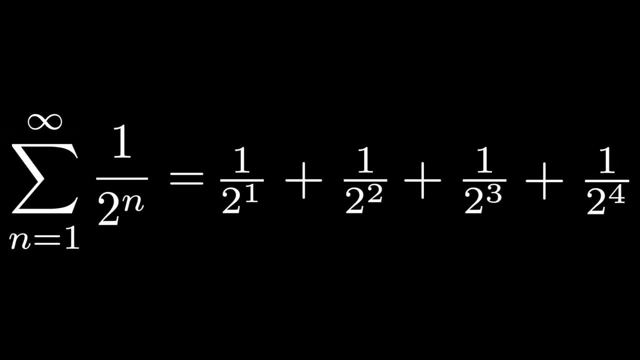 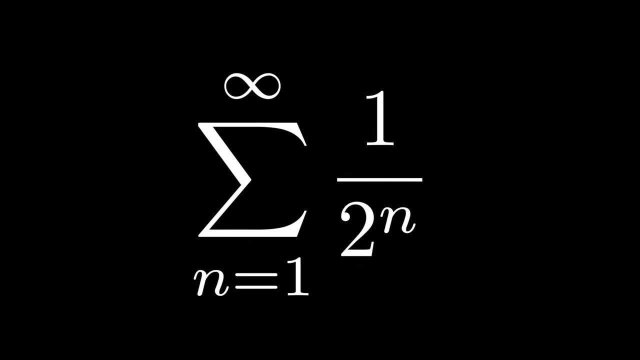 But if you try to add an infinite quantity of numbers together, you'll just keep going on forever and ever, never actually arriving at an answer. What we need is an extended definition of these operations that will let us make sense of infinity in this context. 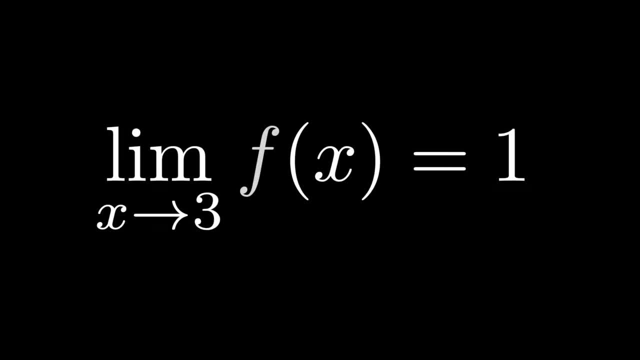 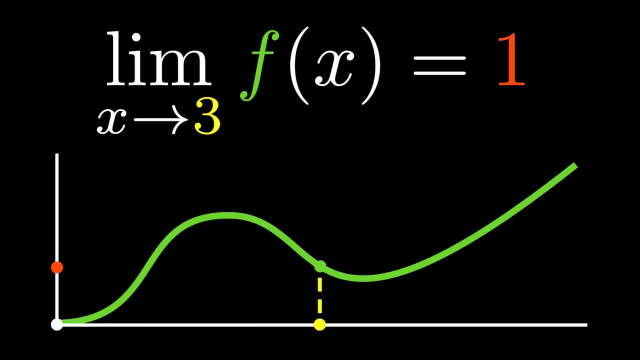 The way we do this is with a calculus tool called the limit, which lets us reason about infinity by only using finite numbers. When a function has a particular limit at a particular input, it says that the closer you get to that input, the closer the function gets to that limit. 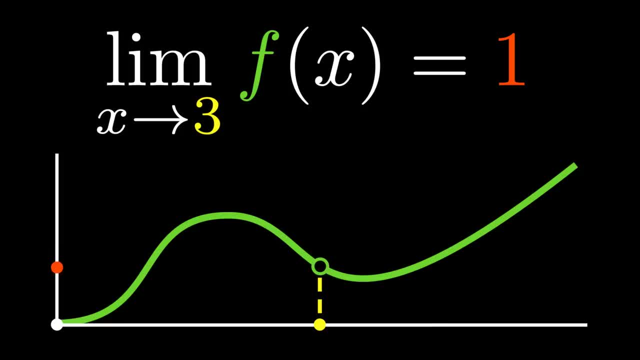 It doesn't matter if the function isn't even defined at that exact point. The limit will just tell you what probably exists there, given the value that's approached as we get close to it. Notice how we can use this tool to analyze points on functions that we can get closer. 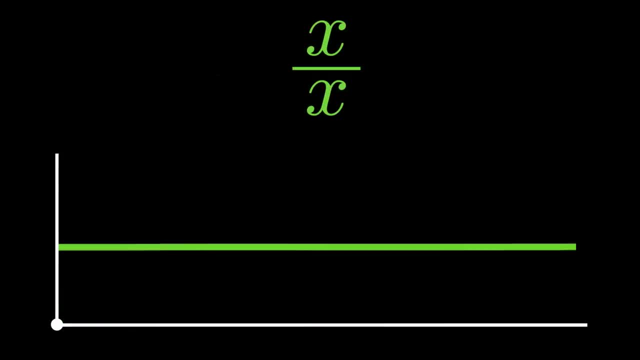 to but not actually arrive at. For example, x divided by x is 1 everywhere except at 0, where 0 divided by 0 is undefined. But if we take the limit when x equals 0, we very conveniently get a value. 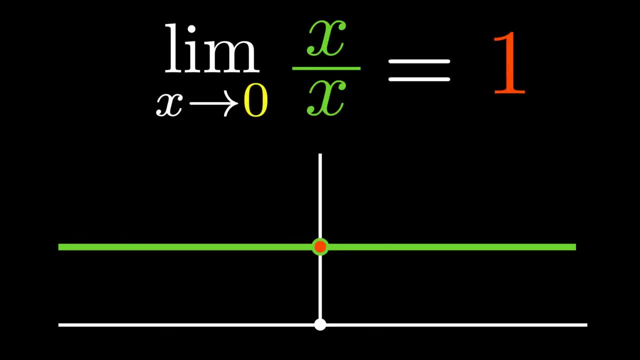 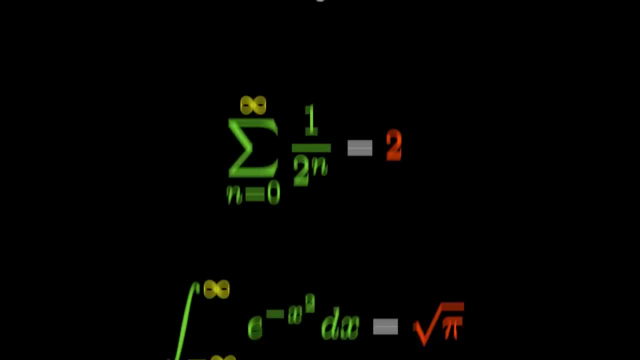 We don't have to come up with a new definition of division to make sense of x divided by x. We can just slap this limit on it and call it a day. Now let's look at those infinite operations again. It would be a pain to make new definitions for each of these operations that say how? 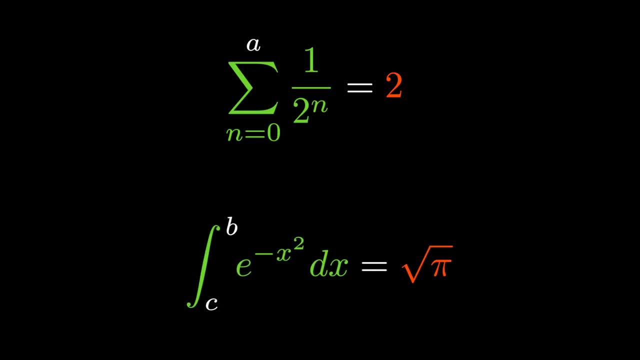 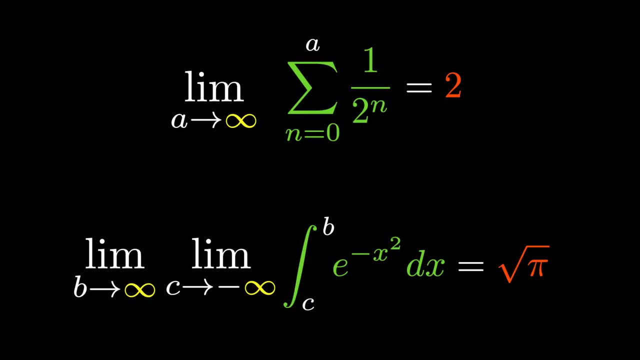 they handle infinities. Instead, we can just use the existing definitions and slap the limit on top of them, Like before. the limit tells us what we get closer to as we get closer to infinity. We'll often skip this formality and just say that the limit tells us what happens when. 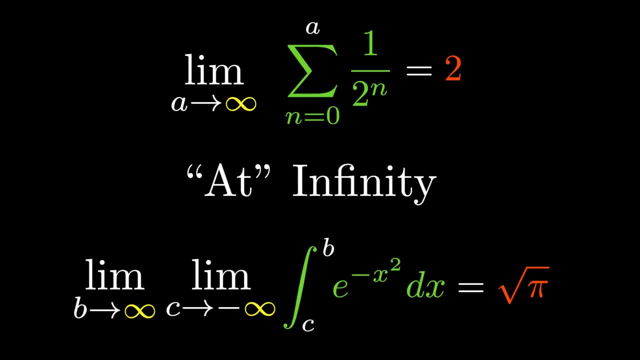 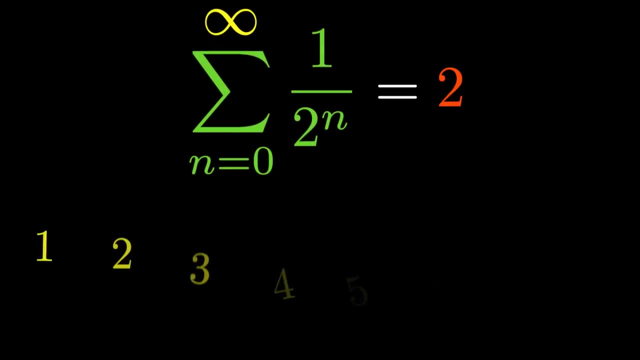 we plug in an actual infinite number at infinity, even though your typical operation doesn't have a sensible definition for what happens when you plug in an actual infinite number. So this equation is really telling us that as we get closer to infinity, the sum gets. 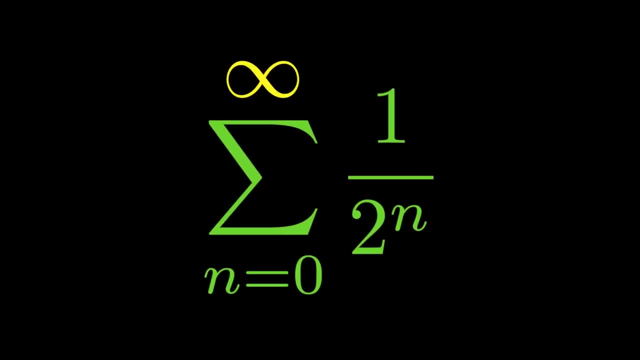 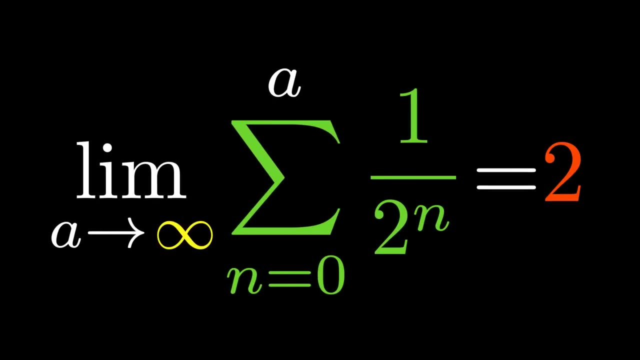 closer to 2.. In summary, it's really hard to directly make a definition for plugging infinity into these operations, So instead we use the limit to check if we consistently approach some specific output as the input approaches infinity. Using this tool, we can plug infinity into all kinds of different operations without